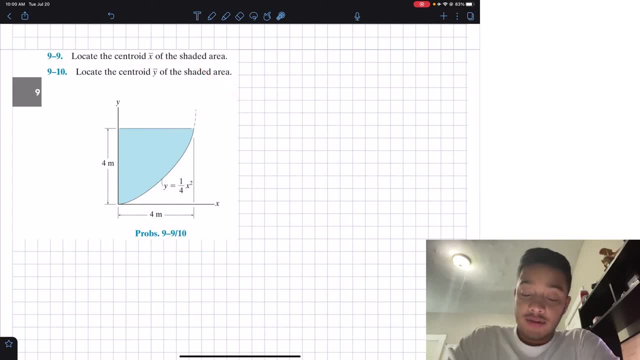 we have this figure now. in the figure we have this y equation that is doing this parabolic shape, and then we need to find what's the centroid of this total area. when x is from goes from 0 all the way to 4.. Okay so let's just start with the first problem, which is problem 9.9.. Okay so, in 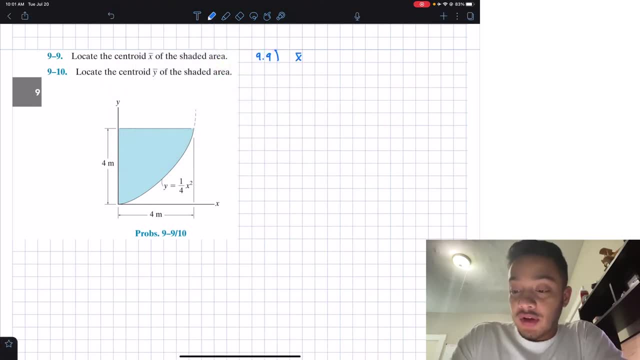 here in this problem. they're asking us: what's the centroid in the x direction? Okay, so the x location. I'm sorry, not the x direction. So in order to find this x direction, we need to find x location. what we need to do is that we're going to apply an integral from an arbitrary for our 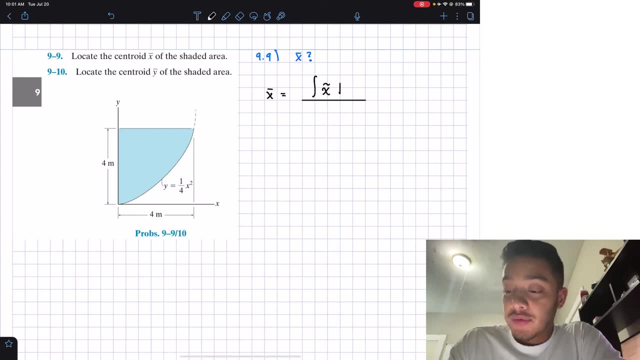 arbitrary summation and the location x multiplied by the differential of my area, and then, at the bottom in the denominator, we're going to have the integral of the differential of the area. Now, in order to solve this problem, we need to find first what's this arbitrary location equal to and what's 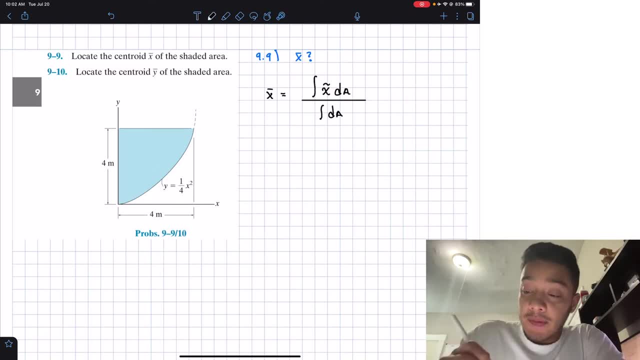 this differential a. So let's start by assuming that our differential area looks something like this, so it should be a really small rectangle right and then our center or our centroid for this differential area, since we know what's what's going to be the center of a square, in this case our differential. 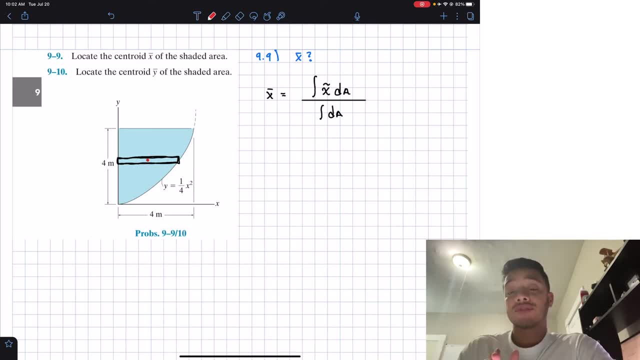 area. it's exactly right in the middle of the x direction and right in the middle of the y direction, so that should be it. that should be the centroid of this, only this specific area. okay, like this specific changing area, so I could have another one here and its center should be somewhere along this. 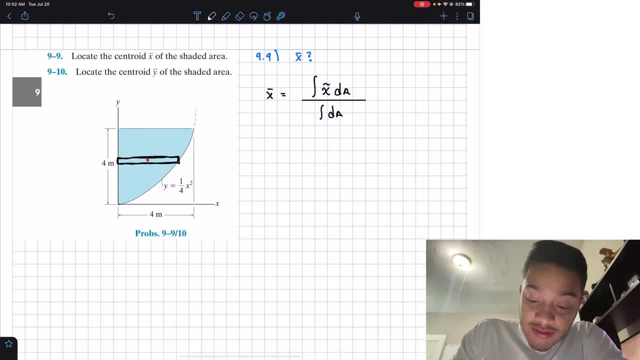 line. now we can say for that, for this differential area, so let me change the eraser. it's too big, so I can just pull this down and find out what the value for that is in my area and we'll go back to the description and I'll show you how to figure it out in a few seconds. So I need to find that out, so we 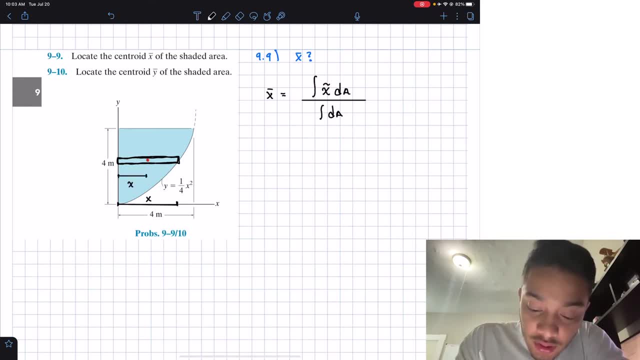 can find that out. so our centroid number two is equal to half of our x. So now let's see our value of x. so where the x is on top of our x, that's aします star and our z is an 8. The z is the center. 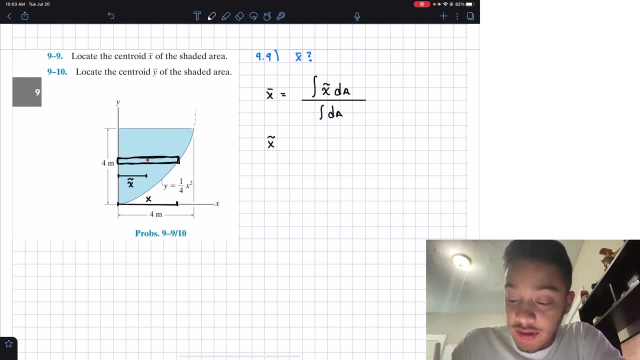 of the x and the point of the z is the point of the z and that's what's going to school. the z is in the center. it's equal to one half of my value of x for this differential area. okay, now the last part that we 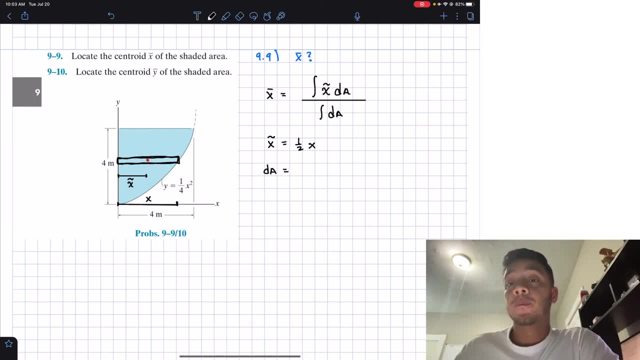 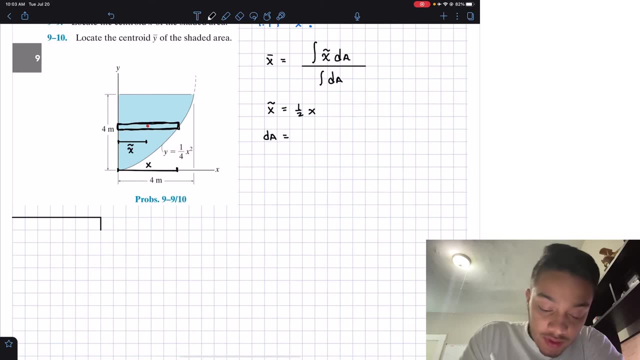 need to find is: what is this differential area equal to now? if we were to redraw- let's redraw our differential area over here, on our left- that what we'll find out is that over here we have the change in the y direction and then in here we, as we said before, this is equal to my value of x. 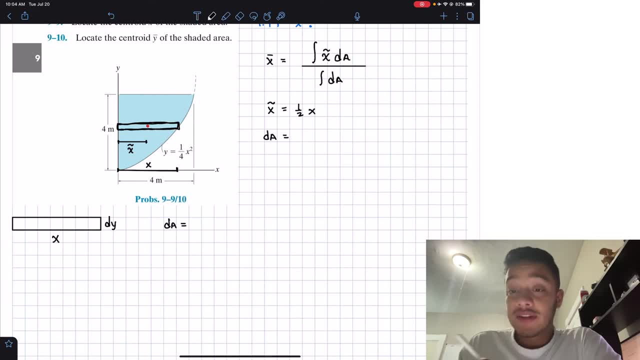 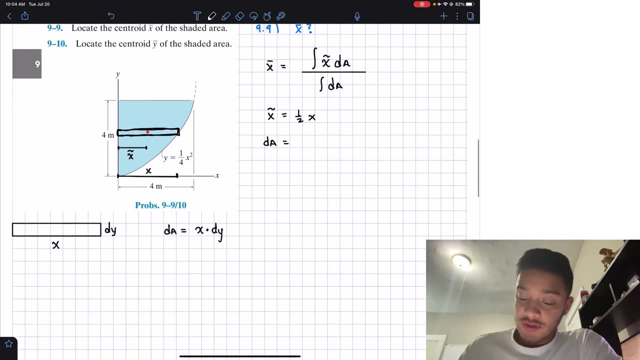 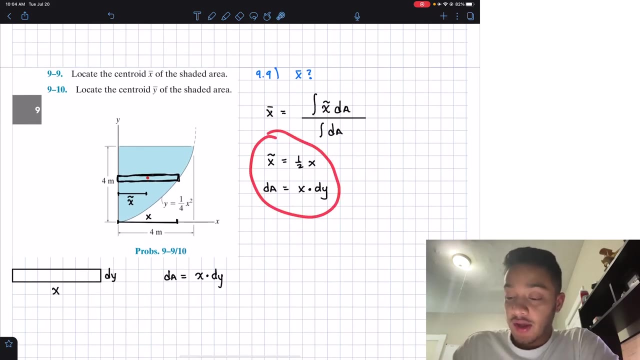 so the area of this rectangle, what should it be? well, it should be x multiplied by dy. okay, so we have that this is x times dy. after finding this, we realize that, okay, this one is in terms of x, this one is in terms of x. but i also have a. 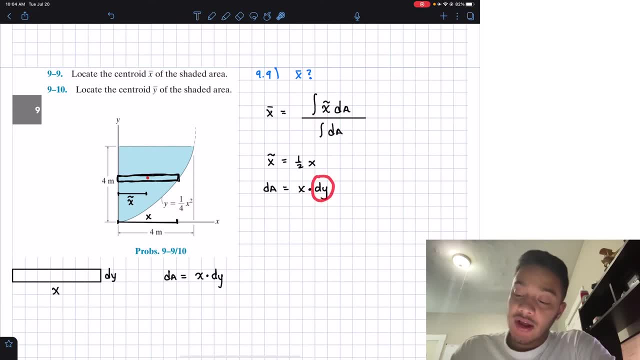 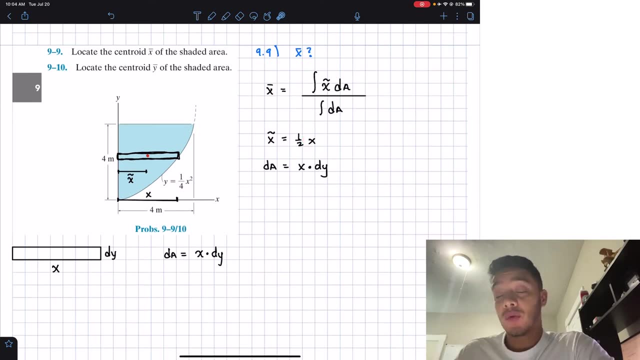 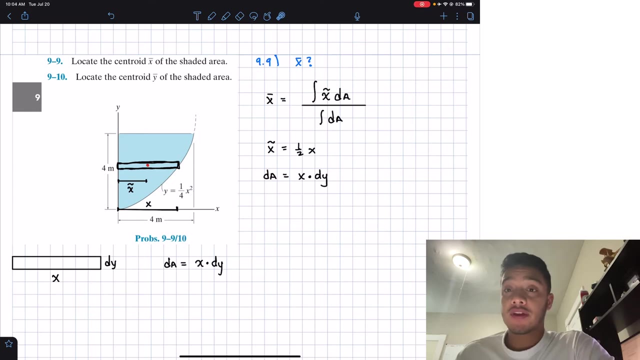 a dy in here, since i have a dy in here and i don't know what this is. what we can do is that we can change these x values into y values. how are we going to change them? well, we have the equation of our line, where y is equal to one fourth of x squared. so, knowing that we're going to take 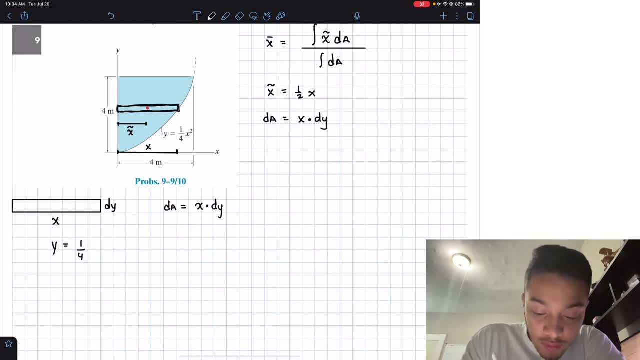 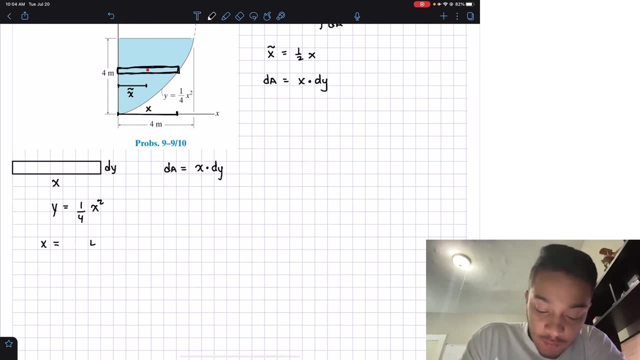 come back here and be like: okay, so y is equal to one fourth of x squared and we need to solve for x. so we're going to solve for x and we're going to have four y, and then we're going to have it raised to the one half, or basically just the square root of four y. we can simplify this also. 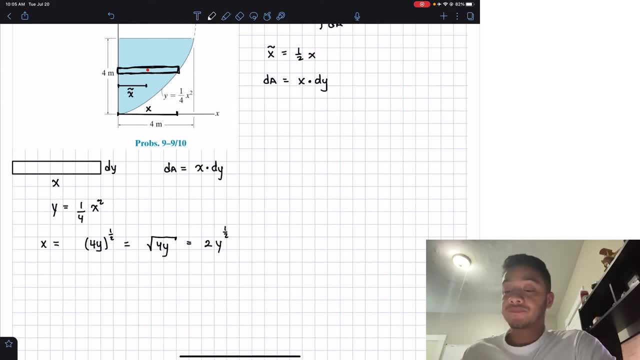 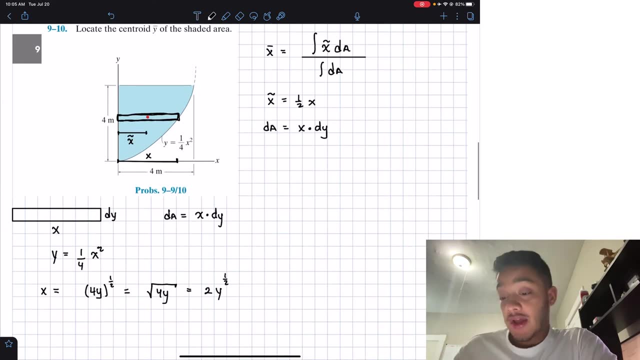 as two y to the one half. okay, which i prefer, um to have everything like this. it looks more in my preference. so now we know what x is equal to two y to the race to the one half. so what we're going to do is that we're going to plug. 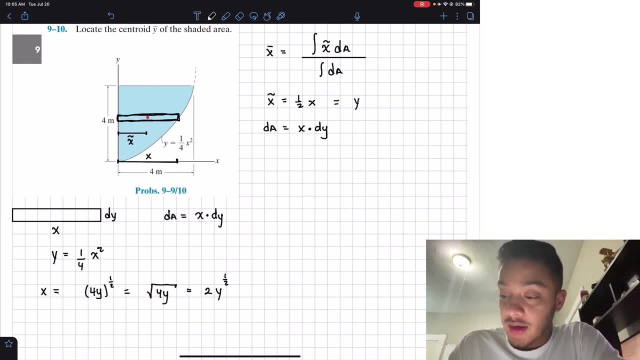 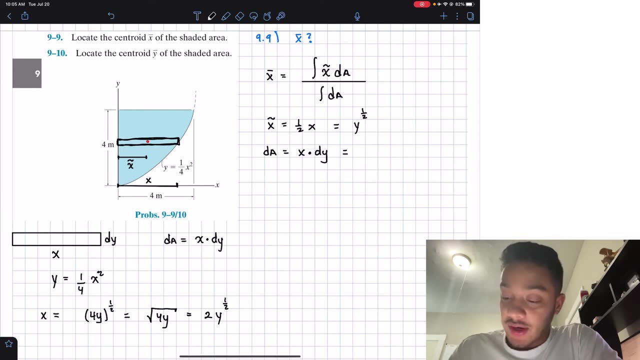 this in here. the two cancel outs and we will find out that my arbitrary x is equal to y raised to the one half and my differential area is going to be equal to two y raised to the one half multiplied by dy, since now all my terms in are in one single variable. 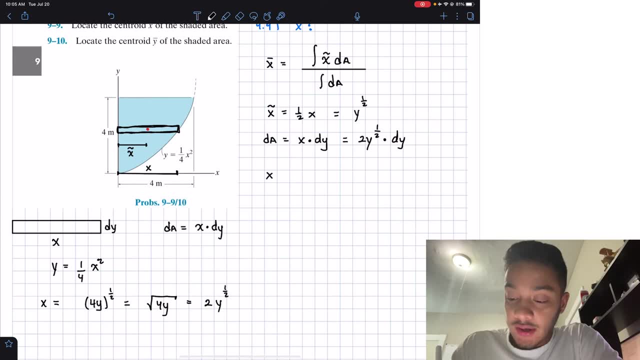 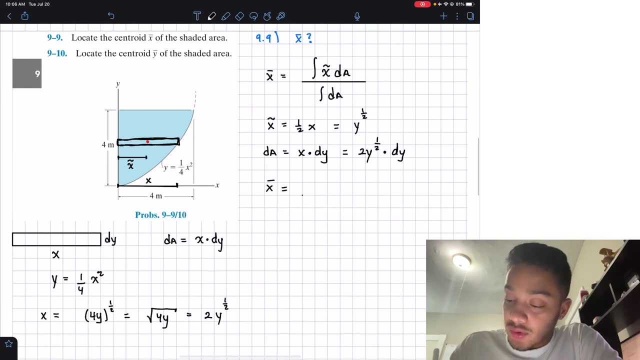 so what we're going to do is just go ahead and find my centroid location, my x location, centroid x location. so we're going to plug in on our integral, which is going to be well. first we have arbitrary x, which is going to be y to the one half multiplied by the differential area which. 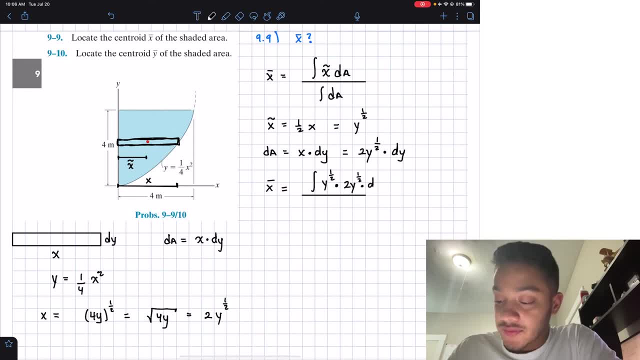 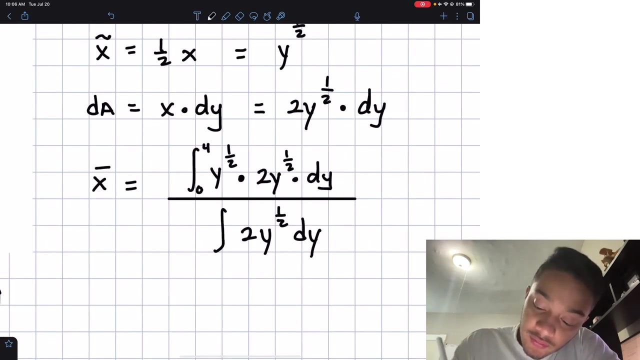 is two y to the one half times dy, okay, divided by the integral of the differential area. so two y to the one half dy. now the boundaries are for our differential in the y direction. therefore, the y goes all the way from zero, all the way to four, okay, so we're going to have that on our boundaries. we'll have from zero to four and from. 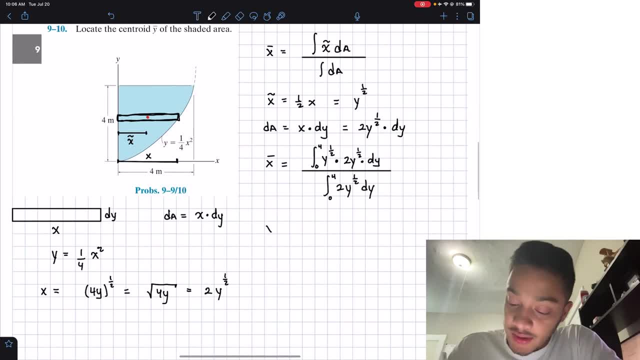 zero to four. now the next thing that we can do is that we can plug this integral into our calculator, so what we have in here. so we're going to do the integral from zero to four, of y to the one half times two, y to the one half times dy, and our numerator will be equal. 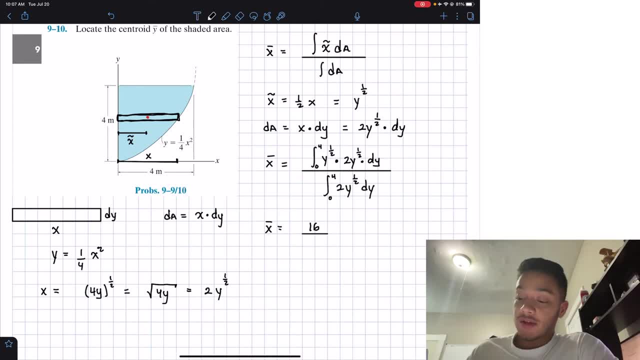 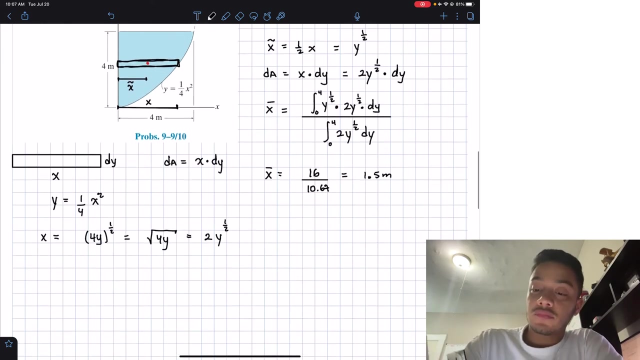 to sixteen, and then our second integral, which is the integral from zero to four, of two y to the one half dy will give us an equal of ten point sixty-seven. okay, now, if we do this fraction, we'll find out that my X location is 1.5 meters and 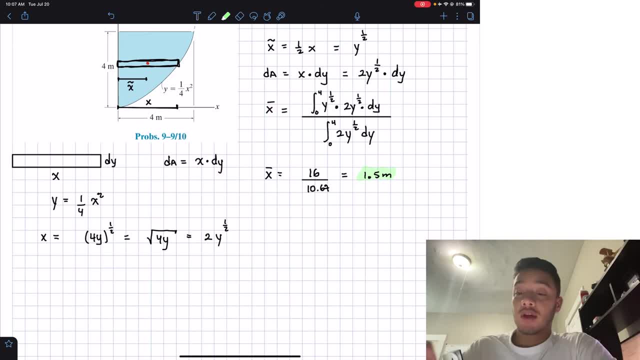 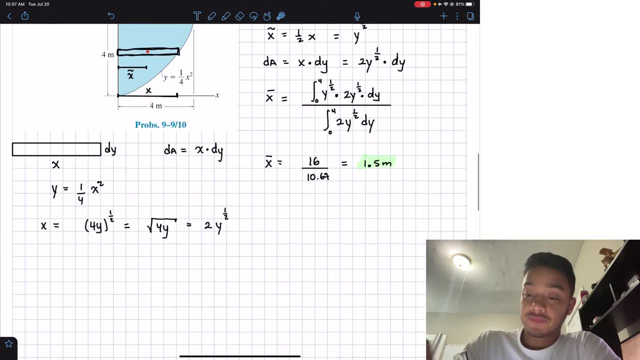 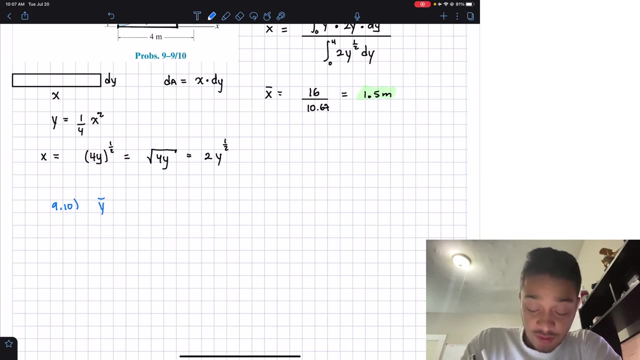 we just solve problem nine point nine. okay, so the next thing that we are going to do is that we're going to solve problem nine point ten. so for my problem nine point 10, they're asking us what is the centroid location in the y direction? and we're going to do a similar. 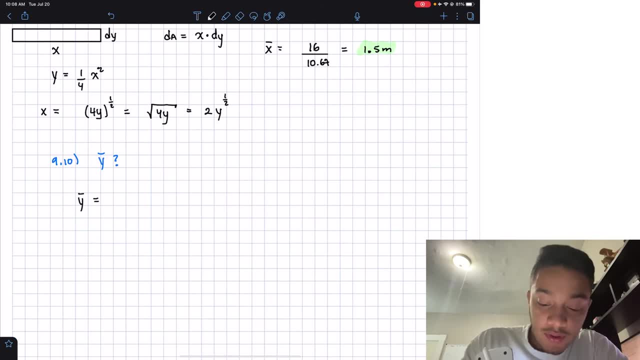 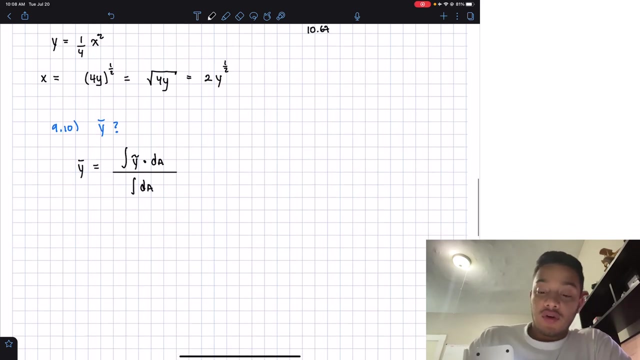 process where we're going to have that. the centroid in the y location is going to be the integral of my arbitrary y point times, the differential area divided by my differential area. so what we need to find is this arbitrary y location, because we already know what the 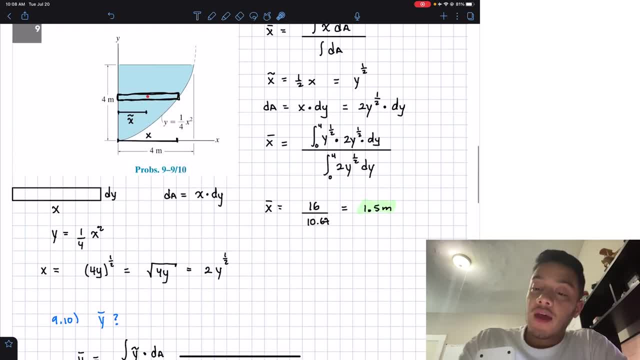 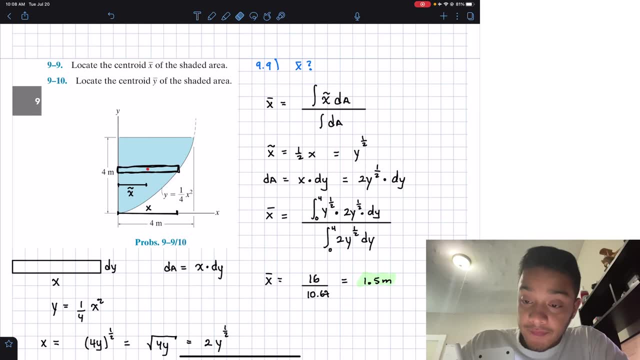 differential area is the a is. so let's go back to my main figure in here and find out. okay, so the value of y for this differential area, so for our square in here, is this one. it's from here all the way from the zero line. so this is my value of y. but wait a second, this is also the value for my. 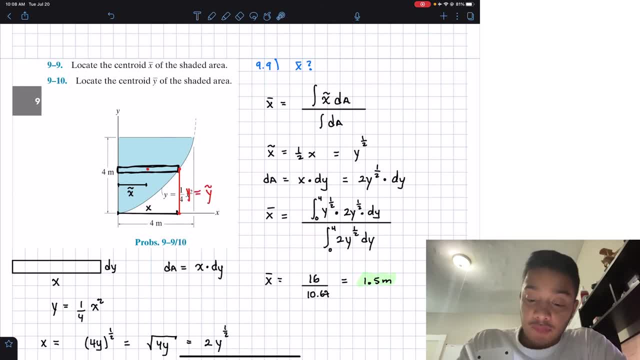 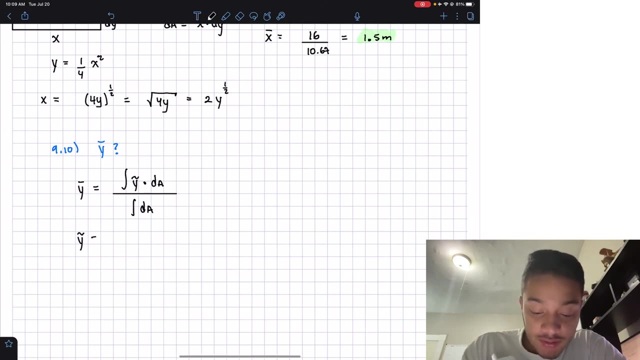 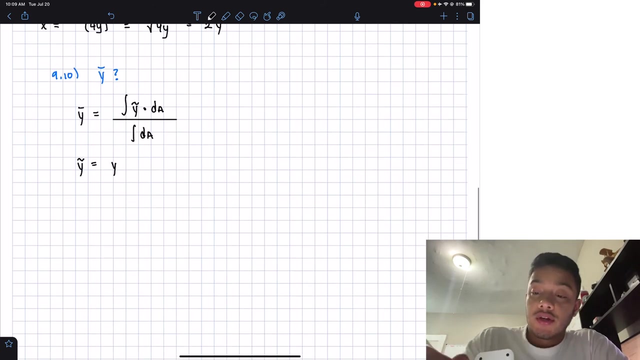 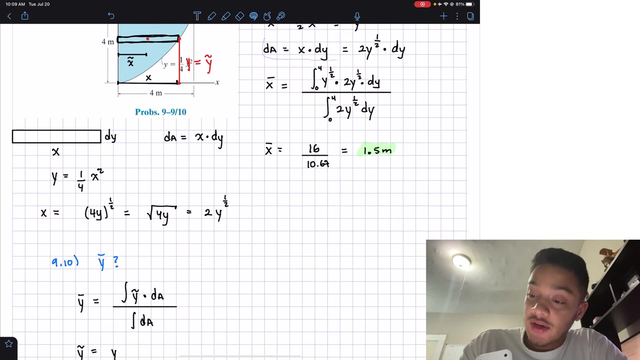 arbitrary point, that is, the centroid of this area, of this differential area. right, so since they are the same, we're going to say that our arbitrary centroid will be equal to my value of y, now that we know this, and we also know from the previous problem that my differential area is equal to this. 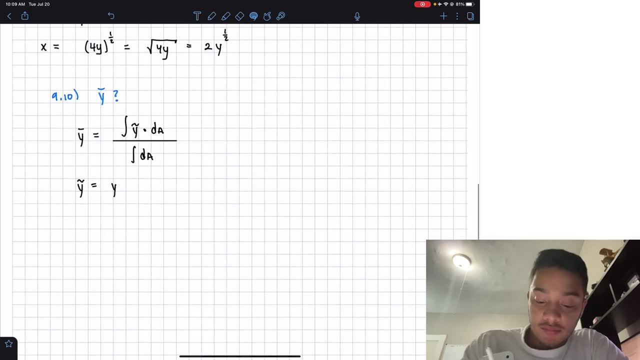 so let's copy it down. so we're going to copy, we're going to paste it in here. okay, so we have our values. so what we can do is that we're going to plug them on our integrals. and what do we have? well, we have y multiplied by the differential. 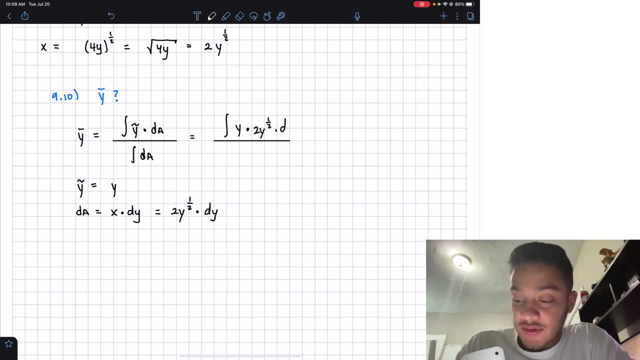 area which is two y to the one half times d y, divided by our integral of two y to the one half times d y, and our boundaries are still the same from zero to four and from zero to four. if we pay close attention, this integral- we did it before- is the same integral as our x location, the